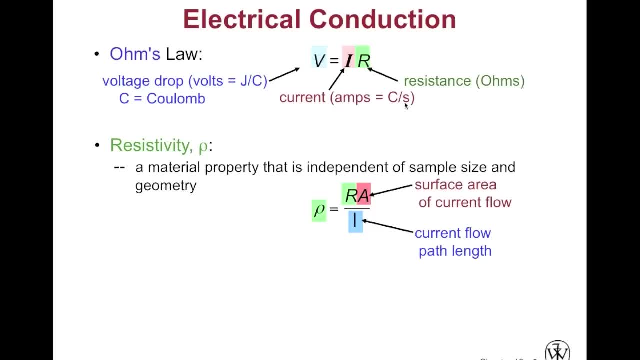 number of column charges passed through that unit times unit. The resistivity is another concept, importance concept. It shows the resistivity of each material and what the geometry factors affect on that resistivity. As you see from this equation here, the cross-sectional area and the length of the spaceman, they both have big effect. 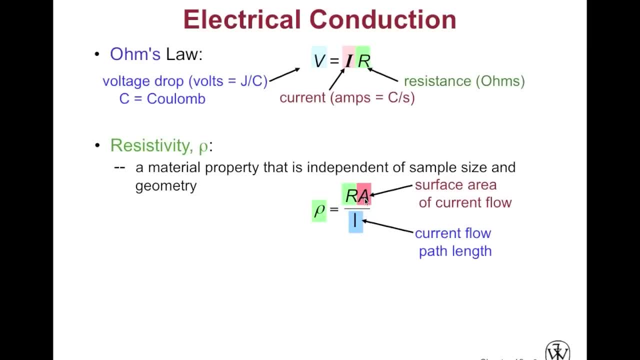 on the resistivity of the material. As we have bigger cross-sectional area and less L, the length of the material, we're going to have less resistance. Conductivity is another important concept which shows how good the material in conducting the electrical currents, which is equal to the inverse relationship with resistivity. 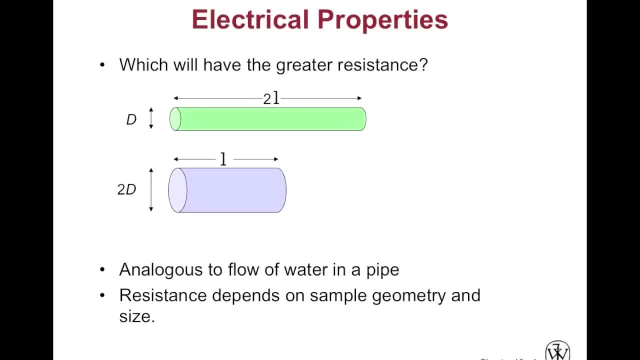 In this problem. we cover that in a class. we show how this two spaceman has different length and different resistance. Subtitles by the Amaraorg community. The two equations here is given. It shows how to find out the resistance for R1 versus. 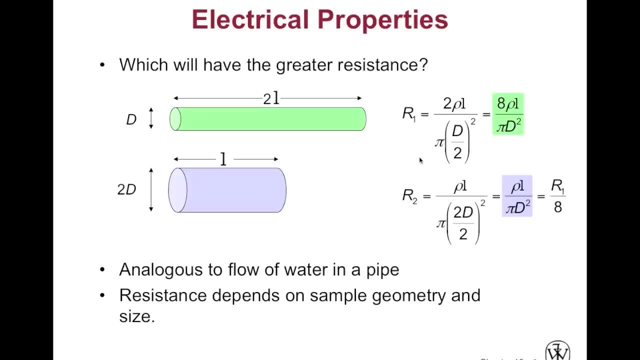 R2.. The question is which one has more resistance? Of course, as we see from the green spaceman, the green one has bigger resistance, The reason why it has longer L and smaller cross-sectional area than the blue spaceman. In this case we can make it a comparison with the water. 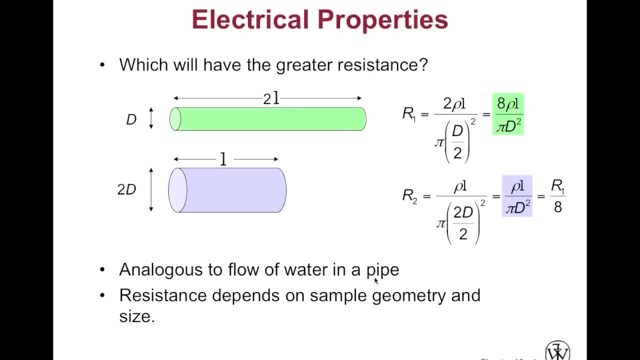 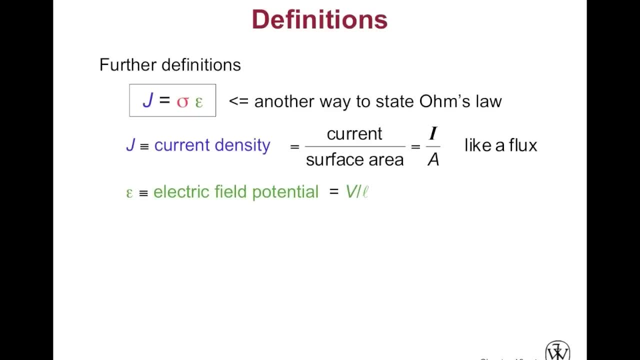 flow in the pipeline. Another important definition is the current density, which shows the relationship between the current and the cross-sectional area for the spaceman. as we have bigger cross sectional area, You're going to have more current density and density is the line yearly L. This means which one has more resistance inاضing 10 times 61% with R1, a 2-layer♥ than A10, or R2, 4-layer♥, Whether or not R1 and R2 blessing a cross sectional area or not, relatives and 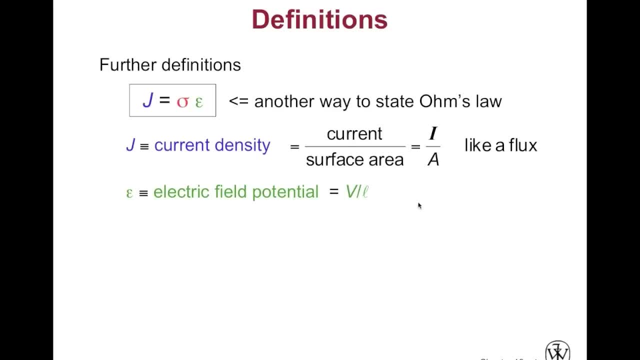 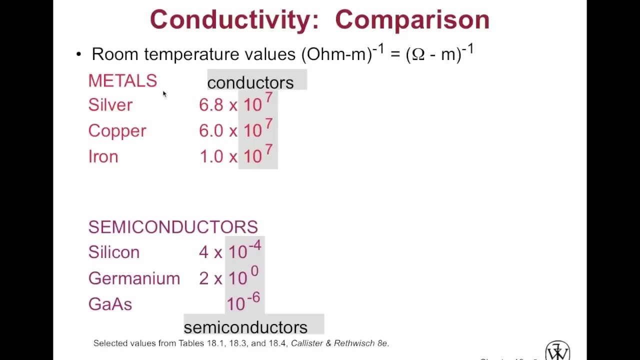 current flux go through that spaceman. another concept we go over, go over it, which is called electrical field potential, which has big effect on the electronic flux, the current density. as we apply more electrical field with good conductivity material we have more electrons currents will flow through this spaceman. the best material we use it for conductivity is a metals, because 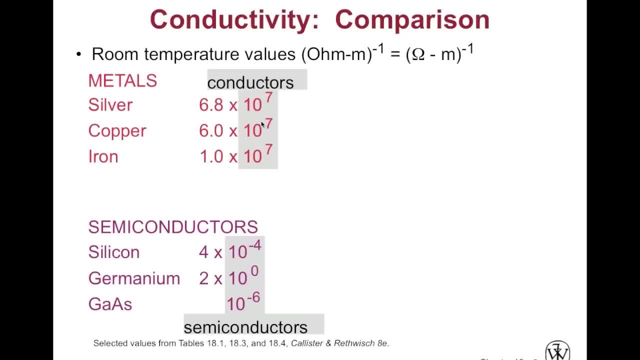 this has higher conductivity and we're going to all go over about it, why it has better conductivity. second, one second materials. it is semiconductor. we use typically silicon and germanium for the conductivity in sensitive electronic devices and how we're going to treat these materials- semiconductors. 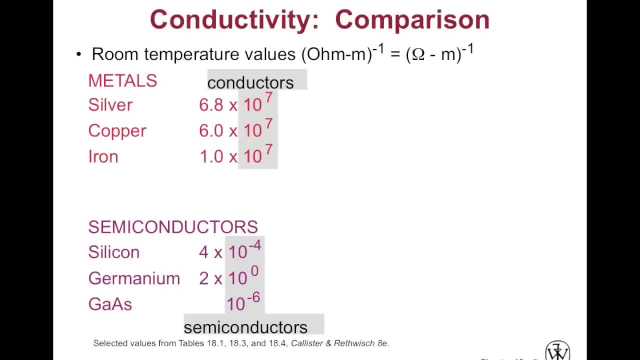 and which make it a higher efficient material for conducting current Ceramic and polymer. there is less chance to use ceramic in our conduction material because their conductivity is typically much lower than metals and semiconductors, While for polymer, as we see here, the conductivity is very. 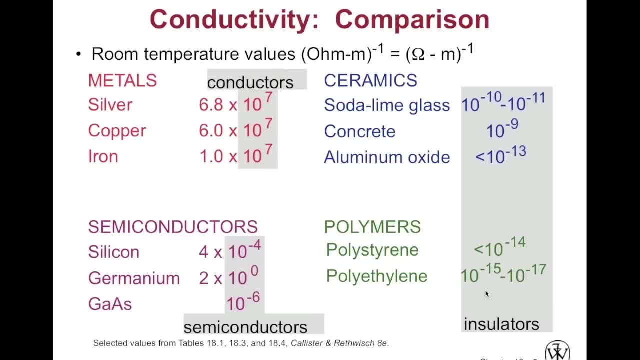 low and we need a lot of big excitement energy to excite the electrons from the valence band to the conduction band and while we apply this energy, this polymer material might burn out before we reach to a conduction band. As an example of 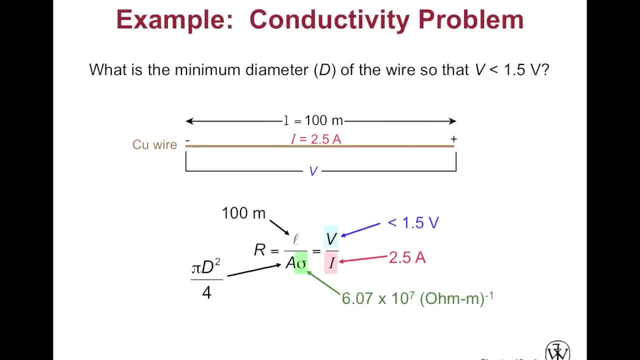 the conductivity for this wire. it's made from copper, which is what typical wires made: from copper. We ask us to find the minimum diameter for this wire if we have applied voltage less than 1.5 volts. As we said in this problem, typically we use 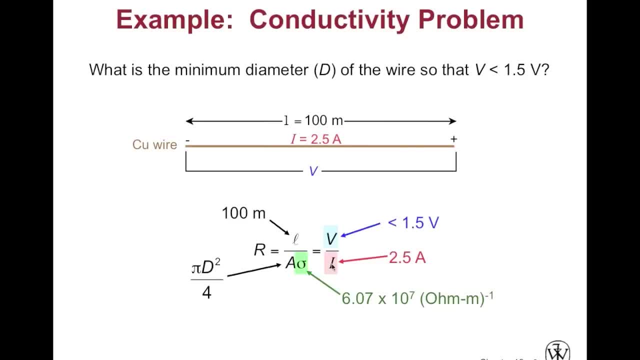 Ohm's law, voltage divided by the current, and if we find the resistance we have to know the length- divided by cross-sectional area for that wire times, sorry, divided by sigma. the conductivity From the textbook table. we have the conductivity for the copper: 6.07 times. 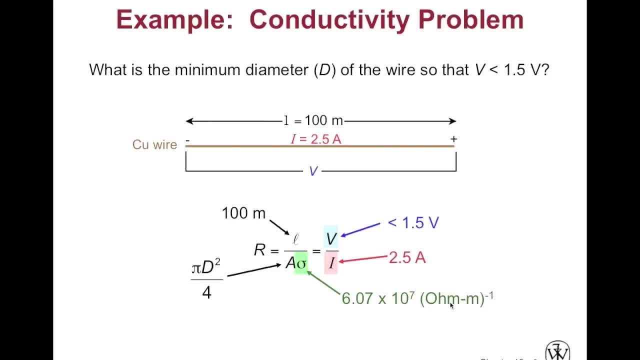 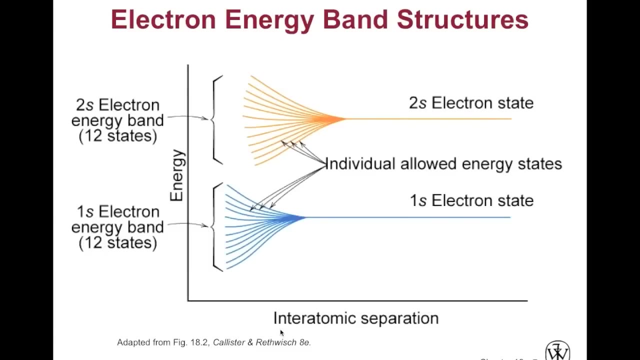 10 to the power 7. so after we find the resistance we can find the cross-sectional area by using this equation. The solution is 1.87.. In all conductors, semiconductors and many insulator materials, only electronic. 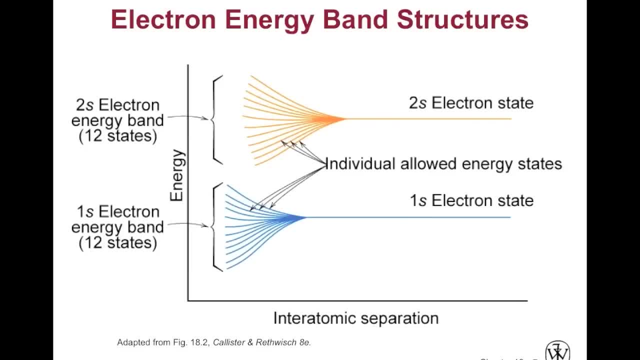 conduction exists And the magnitude of the electrical conductivity is strong, depends on the number of electrons available to participate in the conduction process. However, not all electrons in every atom accelerate in the presence of electrical field. The number of electrons available for electrical conduction 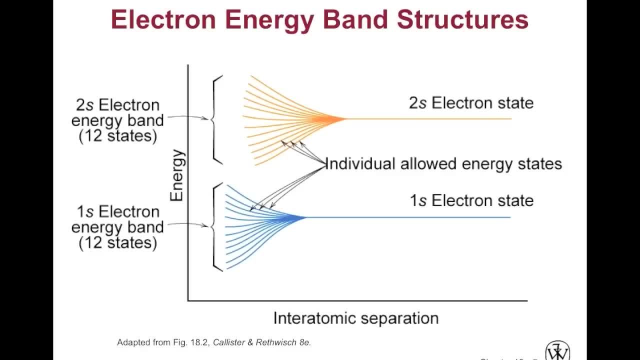 in particular material, is related to the arrangement of electron state or level with respect to energy, in the manner in which these states are occupied by electrons. Anyway, the influence of bangetics is very important. The influence is such that distinct atomic states may split into a series of closely spaced electron states in a solid to form what is termed an electronic energy band. 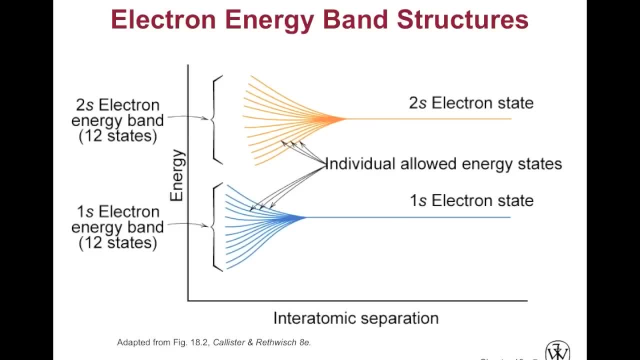 In this schematic plot we show the electron energy versus interatomic separation for an aggregated of 12 atoms. Upon close approach, each of 1s, which is here, and 2s, which is in higher level, atomic state split to form an electron energy band consisting of 12 states. 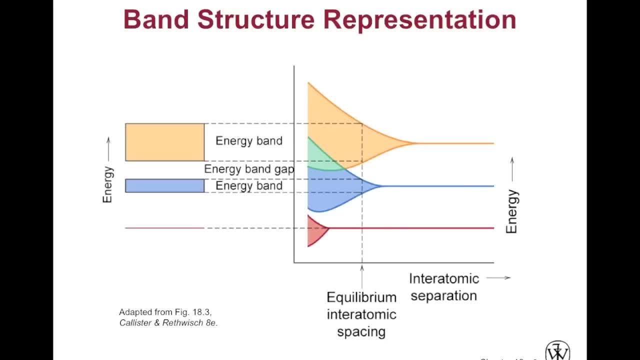 This is another schematic which shows the conventional representation of electron energy band structure for a solid material at the equilibrium interatomic separation. And for this part here on the right side, the electron energy shows the electron energy versus interatomic separation for an aggregated of atoms. 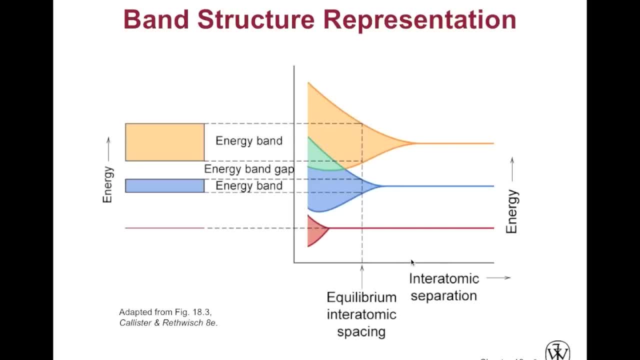 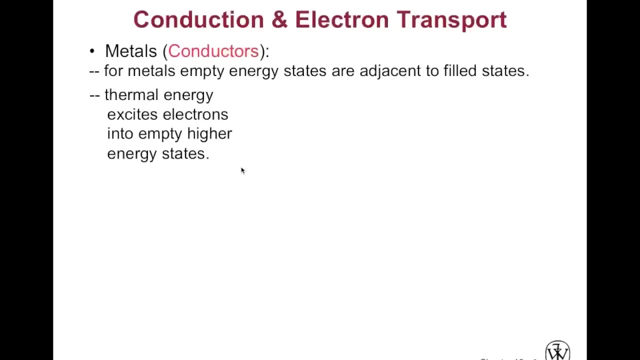 This illustrates how the energy band structure at equilibrium creates amay injection. The energy gap typically is the energy required to excite the electrons from conduction bands to preached band connections, Good connection from arinet band to conduction band. Typically our materials we use, as we said before. 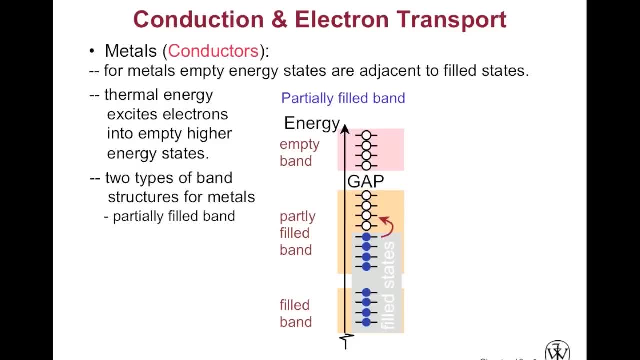 for our conduction. the reason why? because the gap energy interfere with violence band and conduction band in which we need less excitement energy to excite our conduction. correction to excite electrons in our violence band towards the conduction band. anyway, for this schematic it shows there are two. 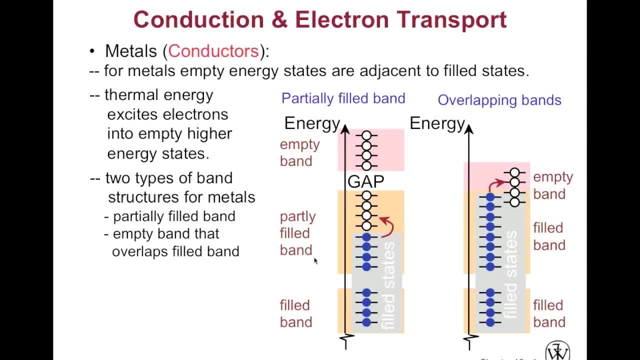 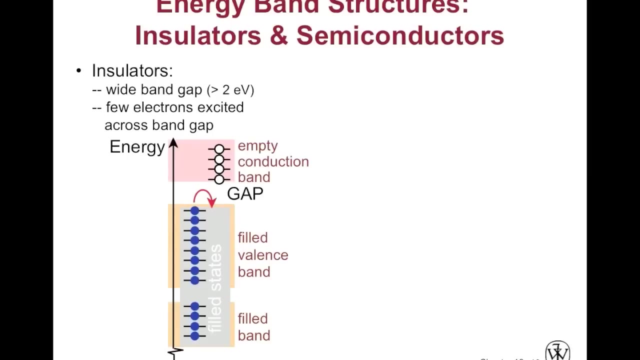 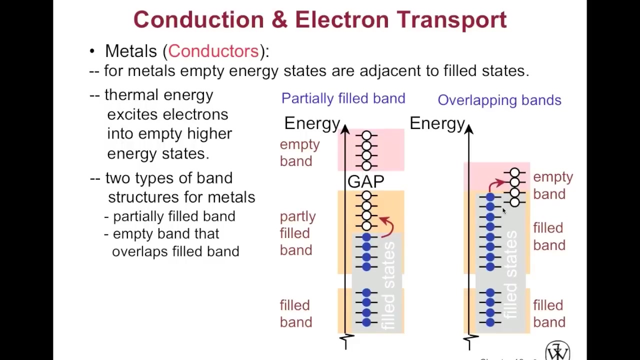 types of band. one called partly filled band, which has some little of free band which need very little energy to excite it. in the conduction band make the material ready to conduct the electrical currents well in second. one second schematic which shows the free ketone already been excited to an empty spot in a conduction band. now 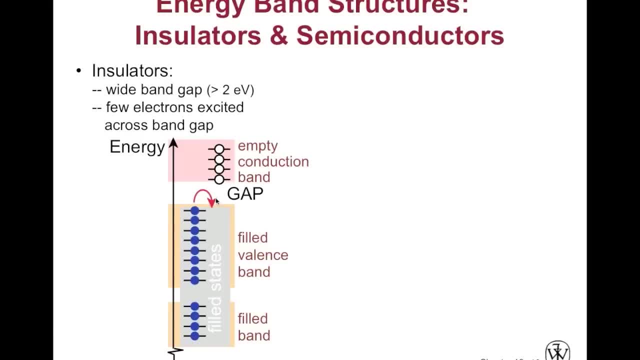 for the insulators and semiconductors we have obvious a energy gap that make a space between the violence band and conduction band. in this case we need higher excitement, energy than metals to excite and free the electrons from the violence band to conduction band. so in increasing the 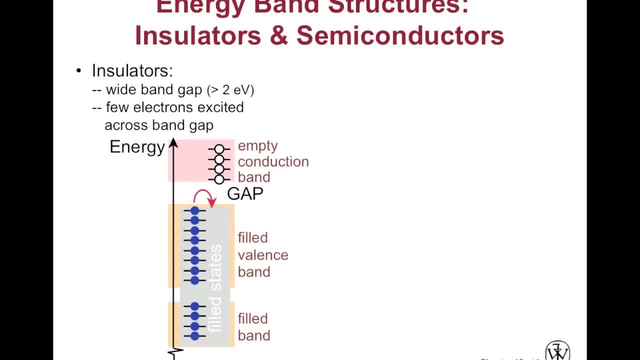 temperature of either the semiconductor of or an insulator result in increase in the thermal energy that is available for electron excitement. therefore, more electrons are promoted in conduction band, which gives rise to gema Bible reserves, 忠祐. in addition, and semiconductor and semiconductor, there is less smaller energy gap than. 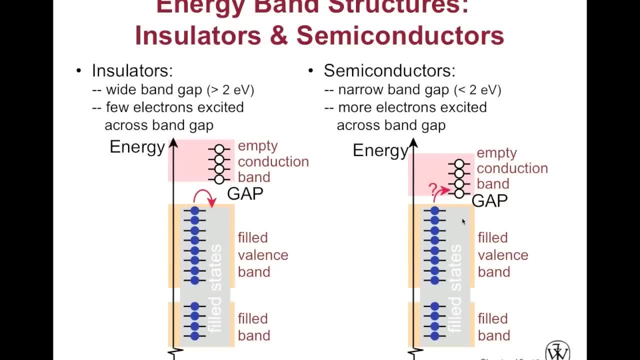 insulator, in this case for semiconductors. we need less than two electron volts excitement energy to promote our electrons from the violence band to the conduction band to promote and get the current charges flow through the spaceman. well, here for insulator we have, we need higher energy gap. 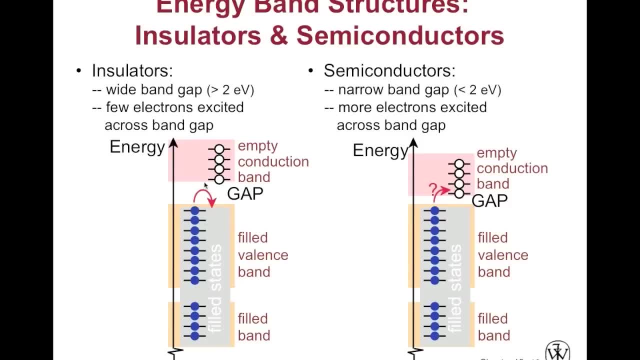 excitement, energy to promote our electrons to conduction band, which typically is not possible to promote our current from the valence band to conduction band, and insulator. the reason why the energy gap is too big to excite our electrons. and the material, insulator material, which is typically 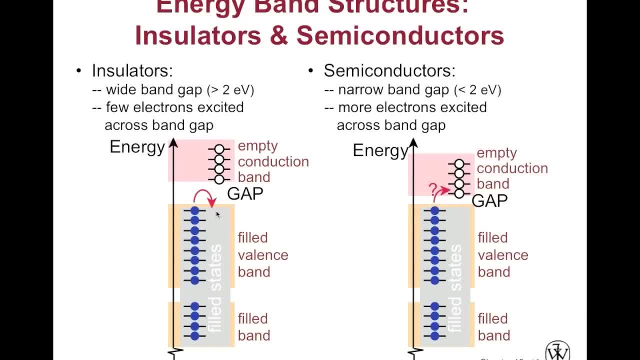 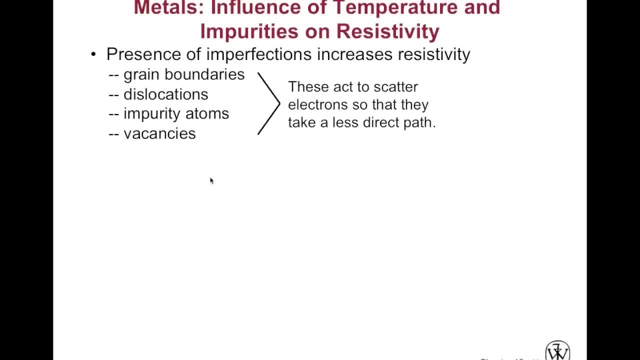 insulator material, which is typically insulator material, which is typically polymer, will burn out before we reach to free electrons. to liberate free electrons in conduction band anyway, there are many factors effects the resistivity of the material. one of these factors called impurity or doping for the 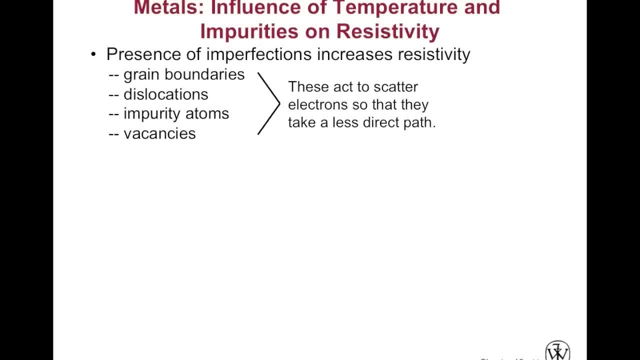 material for specific, specifically for metals, and the reason why, as we impure or are doping the metals, we can make up problems by generating grain boundaries, dislocations and more vacancies, and all these factors will effect on causing trouble, what we call it scattering mechanism. as you see here, from this climatic, when we 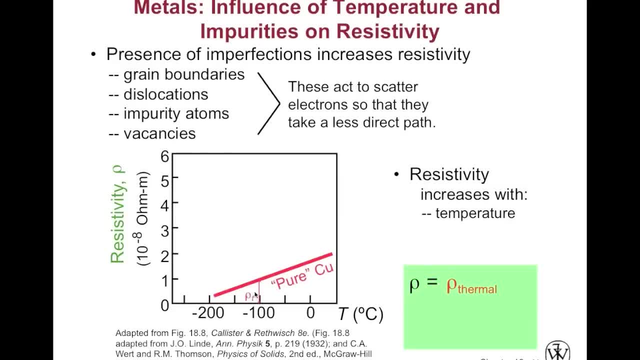 have, your copper has less resistance resistivity. but when we Make it any pure at nickel, The more Density of nickel we add to a copper will have more resistivity, Because the four reasons here will cause this trouble: more resistivity. one is grain boundary dislocation density and the vacancies. and 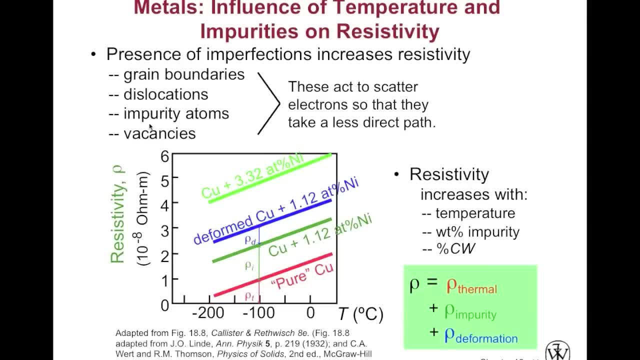 impurity materials, sorry, impurity atoms on all of these will cause Problems for letting current go through more freely in the materials. and This equation here, what we name it, math Heenis rule, if I am saying it right- which shows the relationship or the factor that affect the resistivity of the material. 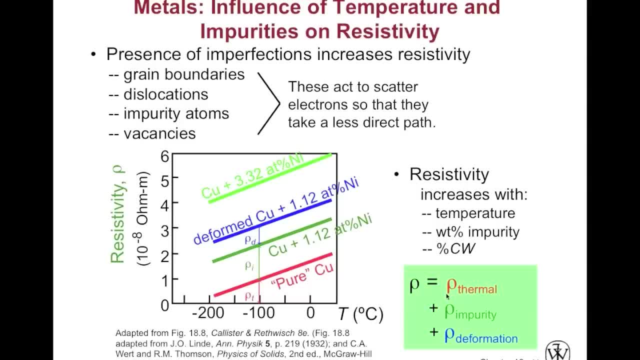 Is specifically for the metals collection, one called thermal problems. the first problem, Which is caused by increasing the temperature, increasing temperature in metals, that will causing a vibration, atomic vibration and atomic structure that will does not make the electrons or Charges to move freely, and that spice man, because that vibration. 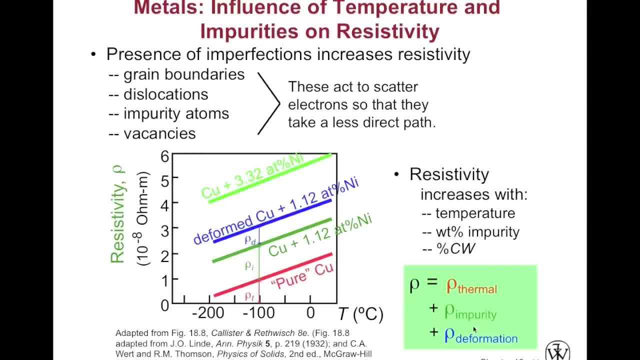 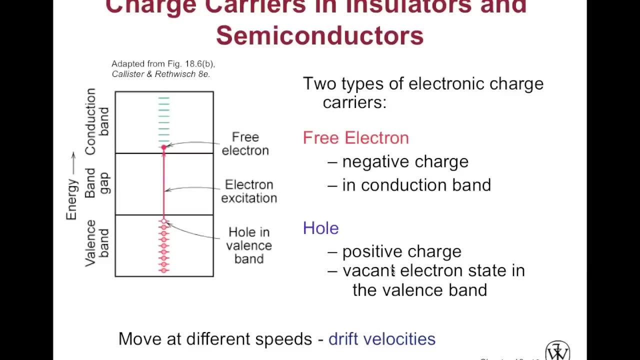 second one, the impurity, as we talked here. and Third one, deformation. as we have more deformation, that will cause or increase the number of electrons scattering dislocations. and this is schematic here, which shows how the Of the, how we excite our electrons from the violence band towards the conduction band. 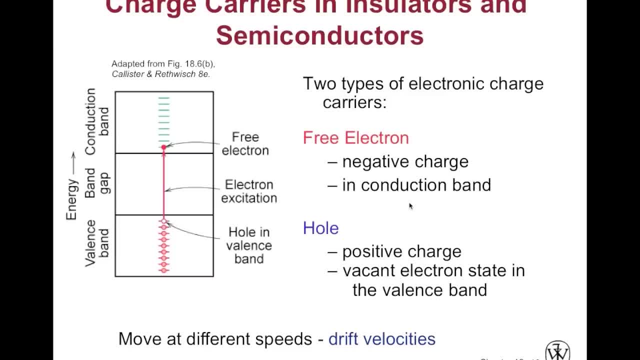 Typically, the electrons has negative charges and they are located in conduction band. That's where the electrical currents will move through the spice man and another method for conducting current, which is called whole, which is generated by Liberating electrons from valence band towards electron band. 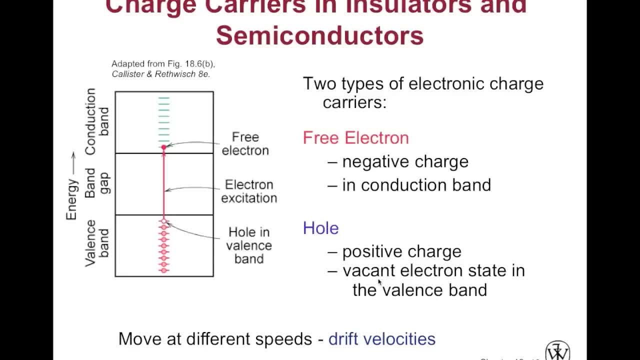 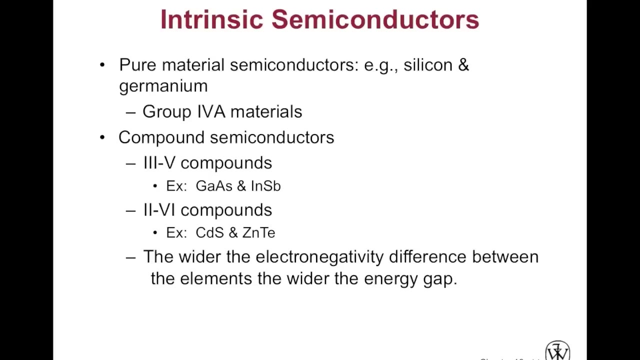 that that will cause a vacant electron state in the wireless band and usually the electron speed is much faster than the whole speed when we apply a electric field. typically in our applications in semiconductor application intrinsic we use silicon and germanium and they are another material we use as a semiconductor. 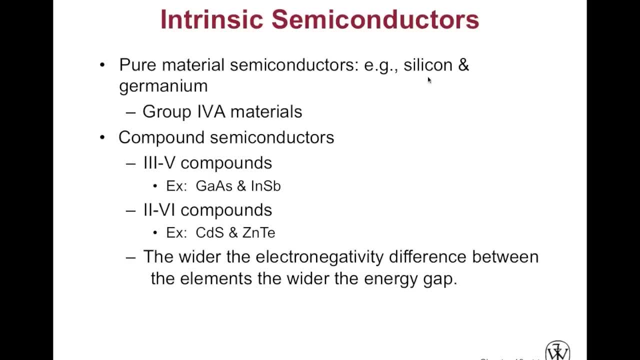 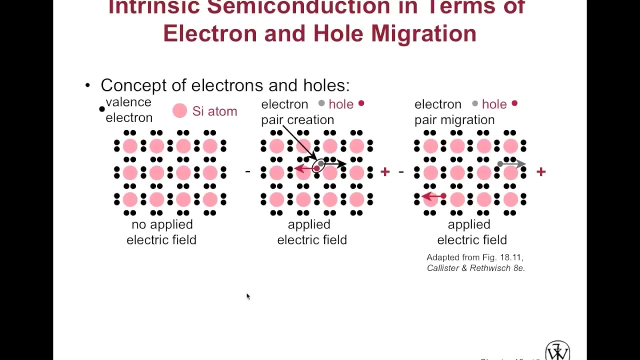 but more usually we use silicon and germanium for semiconductor devices. the reason for that they have wider electronegative difference between the element, the wider the energy gap, as we see here from this schematic, is before we apply electric field and after we apply electrical field, the electrons. 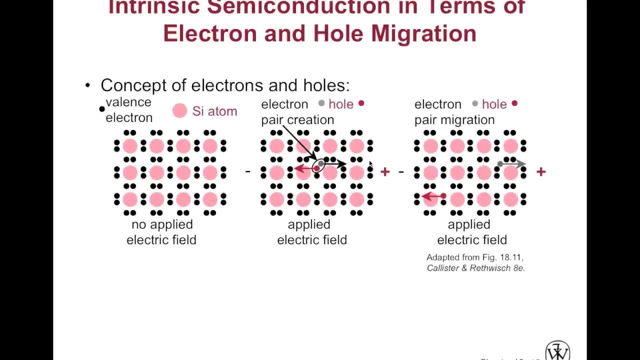 will go to opposite side of the electrical field and holes will go towards the same direction of electric field and the total movement of electrons and holes we call that drift current. this will show the final result after we apply the electrical field where the electron go towards the positive. 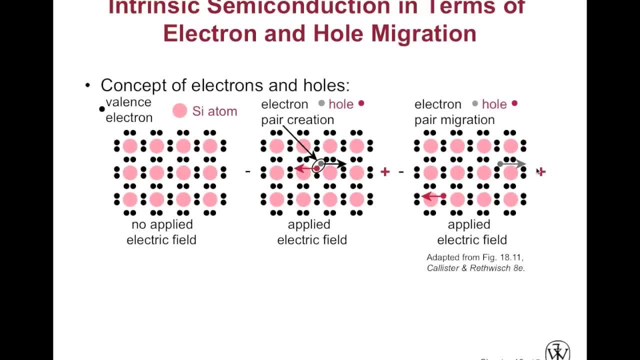 direction of the applied voltage, which is typically the direction of electric field, opposite of direction direction of electric field. and holes go towards the negative side voltage side, towards the electric field direction. here's an important equation. we show the electrical conductivity, the total electrical conductivity for the semiconductor. it depends of the density of 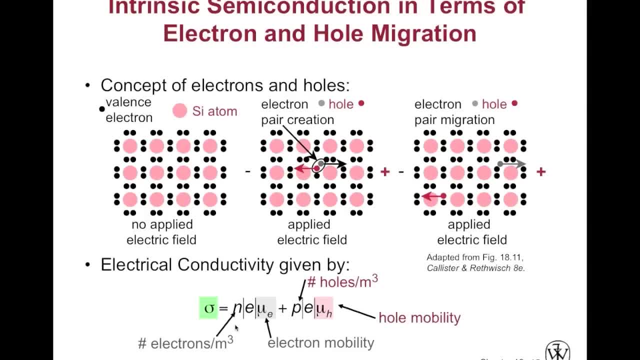 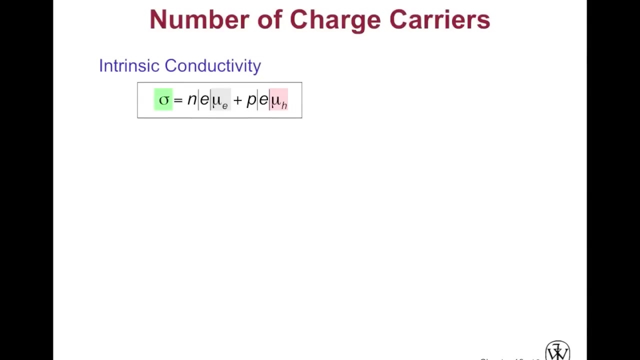 number of free electrons in the conduction band per units meter cube, and p represents the number of density holes per meter cube. and the total of these two terms, which is the mobility for electrons and mobility for holes, will make how good the material: semiconductor material for conduction, current for intrinsic. 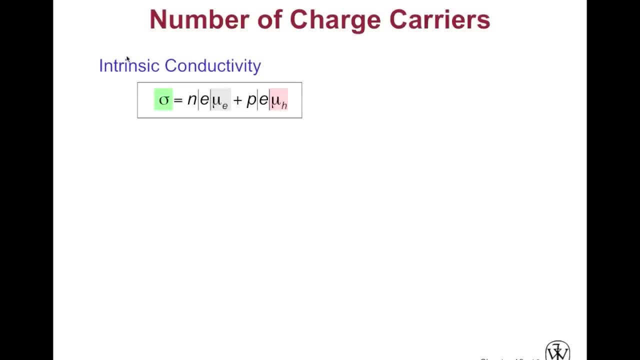 conductivity, this terminology, use that without doping the semiconductor. it shows the relationship again between the density of electrons versus hole and again for intrinsic semiconductor we have number of all equal number of holes. and that makes sense because number of electrons that liberated become originally the number of holes generated. here P is came originally from number of electrons. 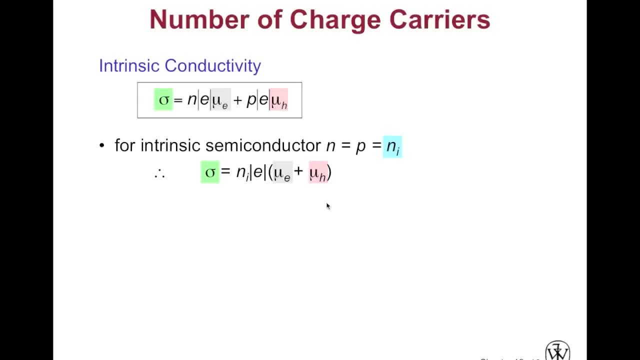 liberated and excited to conduction band. and if P equal N, we're gonna have this equation, which is specific for intrinsic conductivity, and this equation here we asked us to find the density for number of electrons per unit, number of holes, unit volume. after we apply this equation for GAAS, the conductivity we have units. 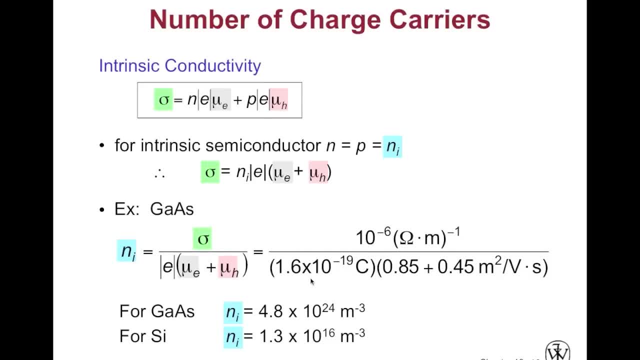 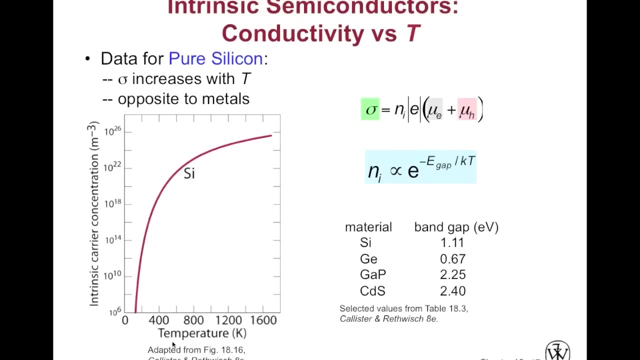 for this specific material: 10 to power minus 6 on electron charge E 1.6, 10 to power minus 19 and, as we said before, the mobility for electrons is higher than mobility of holes. after we apply this equation, we could find out the density for GAAS, and same thing we can use it for silicon. so 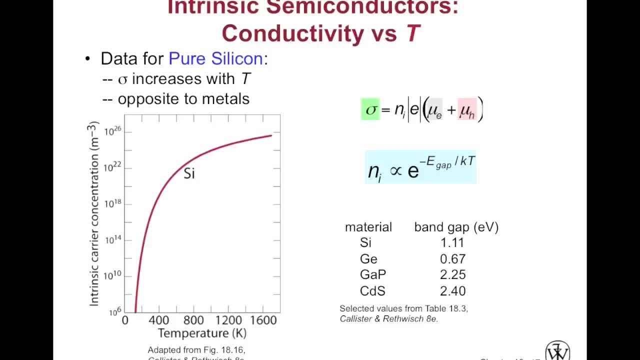 what's the relationship between the temperature and conductivity and semiconductor? for metals, the temperature make the resistance or the sensitivity of material higher, while or where else? for semiconductor, the increasing temperature, while. increasing the temperature making the conductivity is better with less resistivity. the reason why this temperature T will increase the number of liberated electrons and which has an 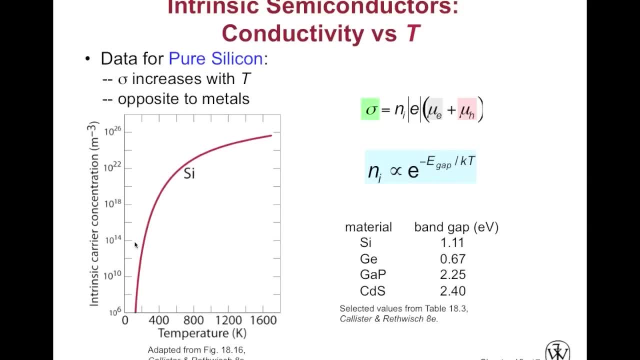 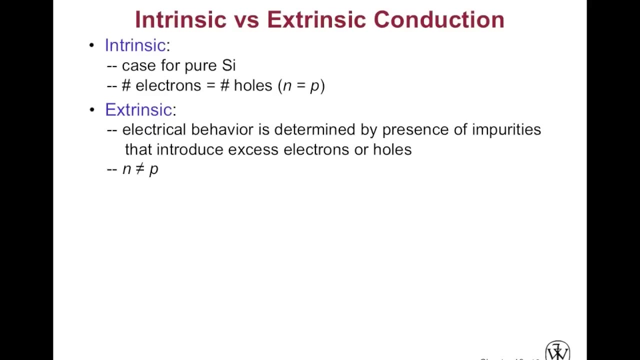 exponential relationship as we increase the temperature when increase the number of concentration liberated electrons. on other hand, we have a terminology called extrinsic, which is came originally by doping the materials, the semiconductor materials, with another material which make the temperature. and our challenge, brought by doing pranking with these methods, is: we can 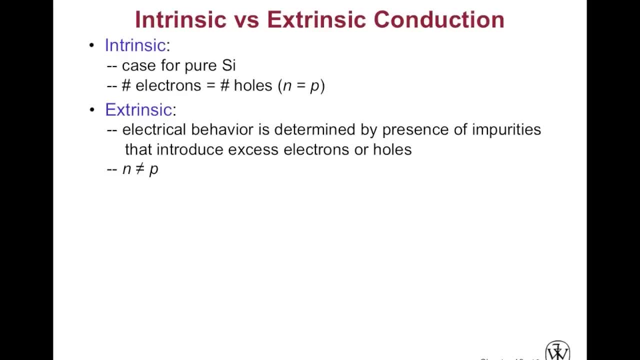 crystal and you can see the呱. and we did an experiment also, we used the neural network. we did a damage 2018 and you will pay what bad the aluminum exotica played the bigger gazelle-sized males in theników that value in the meter, so f? nada good. 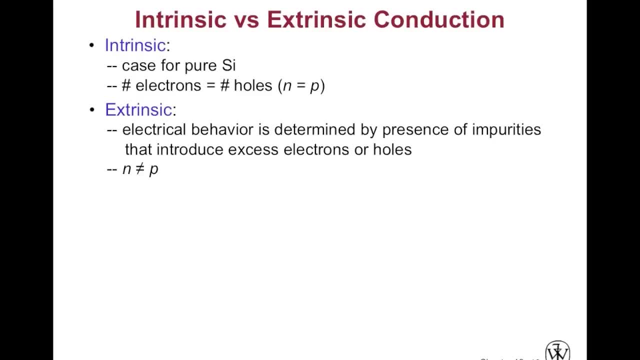 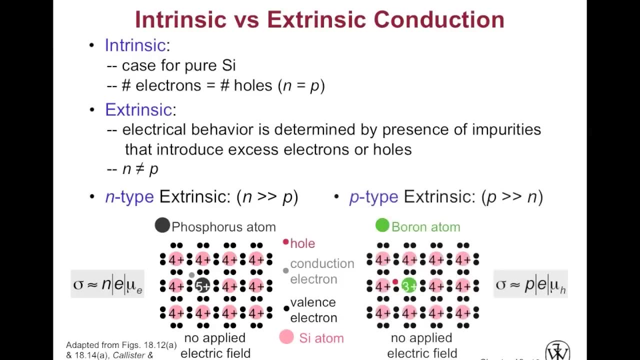 that is what's the answer if you apply the canonical process of emission to the electrons towards the conduction band. As we see here, we dope this semiconductor material with phosphorus atom. The phosphorus has five valence bands and in this valence band we have extra electrons. 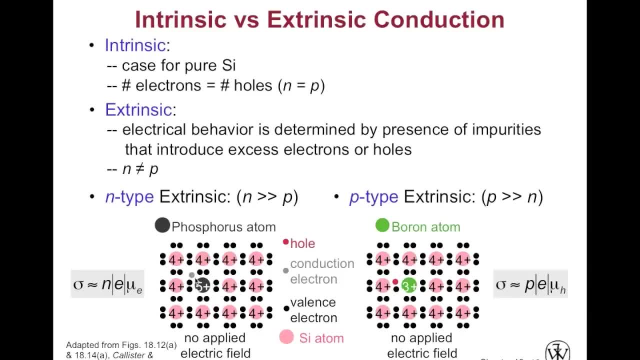 So this electron will be closer to Fermi's energy level and make it much easier to liberate these electrons towards the conduction band. I make the semiconductor Higher efficiency in conduction. Well boron we have in p-type extrinsic semiconductor. 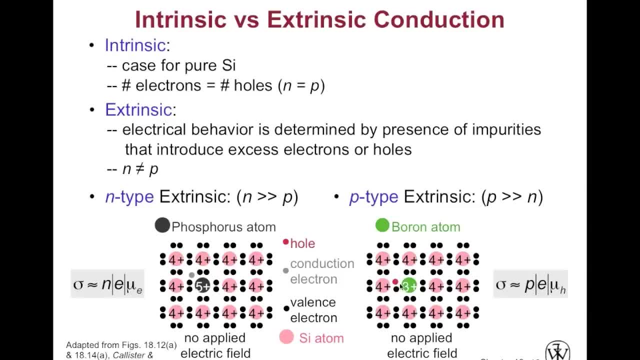 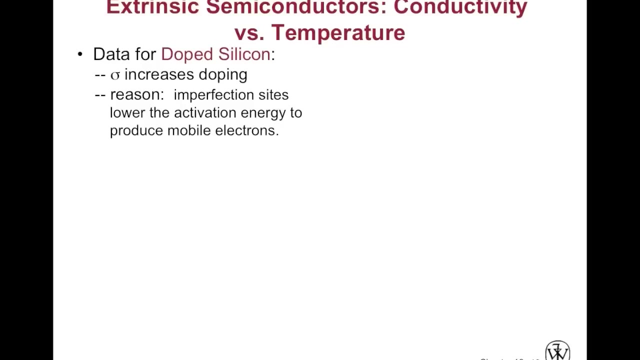 We have one empty spot, what we call a hole. We can use this hole for conduction, which is also close to Fermi's level, and this hole will play a big role- And a few holes For conduction and semiconductor in higher efficiency. 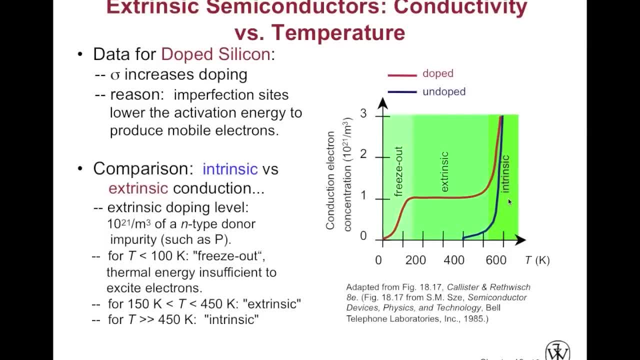 Again to make our comparison between extrinsic and extrinsic material in terms of the applied temperature. So for extrinsic it needs less temperature than extrinsic Because again we dope it With p-type extrinsic, In case we have phosphorus, in case we have N or boron, in case we have p-type material. 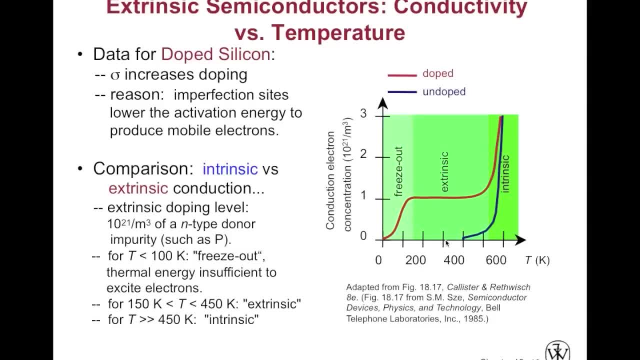 So this guy extrinsic will need less excitement, energy temperature to liberate our electrons towards the conduction band from valence band to conduction band. So in this case for doping Doped silicon, we have conductivity increased with doping. 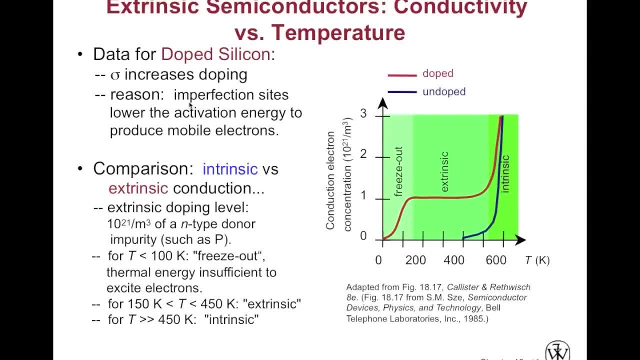 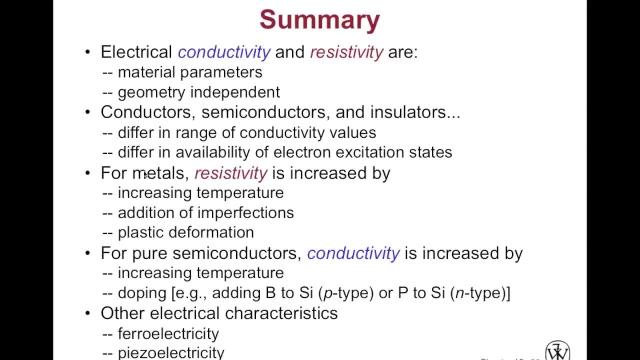 The reason why, as we said, as summary, because the amplification site lower the activation energy to produce mobile electrons. As summary for our presentation for today, we have two very important terminology, one opposite each other as inverse relationship. We have two very important terminology, one opposite each other as inverse relationship. 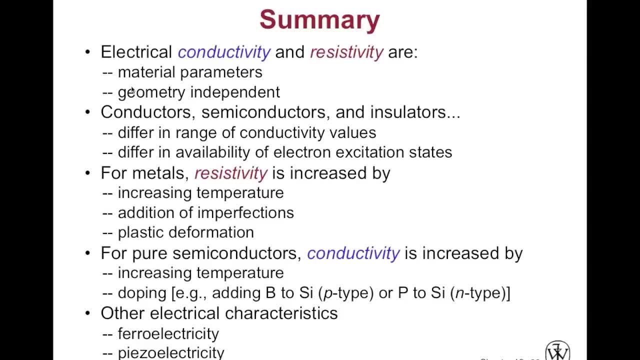 One conductivity called, and the other one resistivity. They both depend on the material parameters, which is, in other words, each material has their own conductivity and resistivity And the other one the geometry, specifically the length for the material and the cross-section. 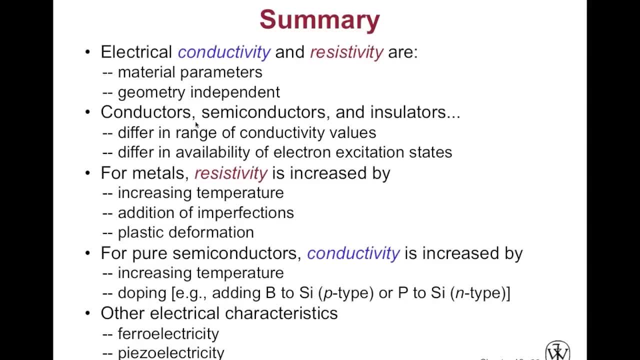 area. We have three kinds of material in terms of conductivity. One is conductor Came from metals. typically We use copper and aluminum for our conduction, despite the fact that silver is also the best one for conduction, but we don't use it because it's expensive. another one is semiconductor, and 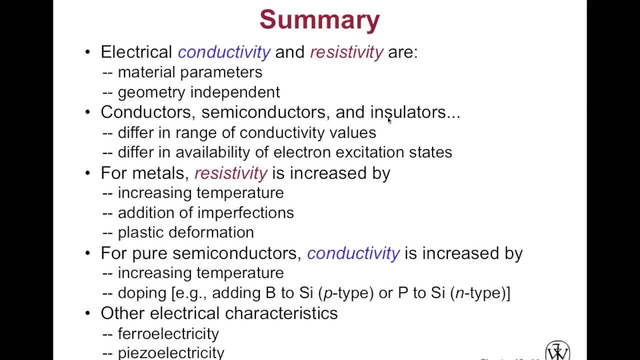 insulator and we make a comparison between these two guys, semiconductor and insulator, and we see the energy gap, the difference between the energy gap between them. for metals, the resistivity increases with the temperature because that will increase the atomic vibration that will impede the current flow through the material, also adding amplification. 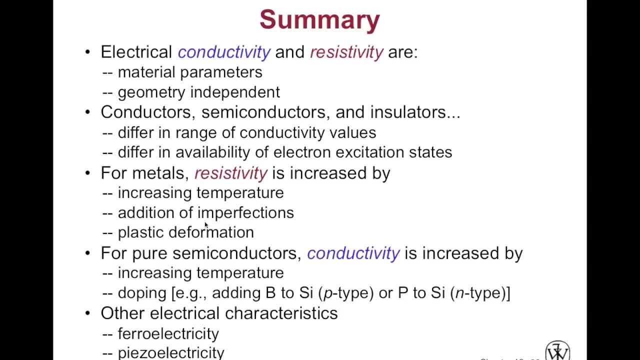 because that will increase the number of grain boundary and dislocation density and plastic deformation will cause the current to flow through the material and also increase the. also more resistivity because increase the number of electrons scattering dislocations. for pure semiconductor we call the intrinsic. the conductivity is increased with the temperature. 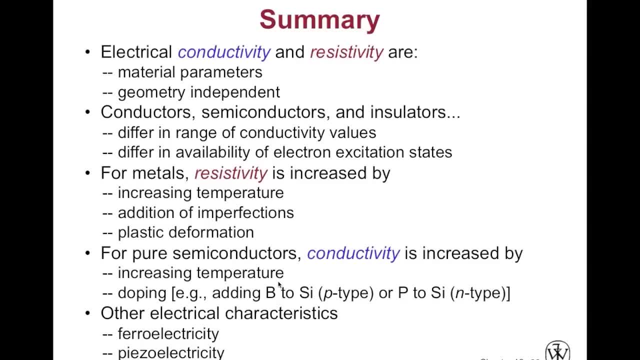 as this temperature will liberate more electrons from the conduct, from sorry, from the violence band towards conduction band, another kind of semiconductor- we call that extrinsic by scattering, but asма is shown that he originally has a very strong field and when we can loops here, for example, uh, some of the past. 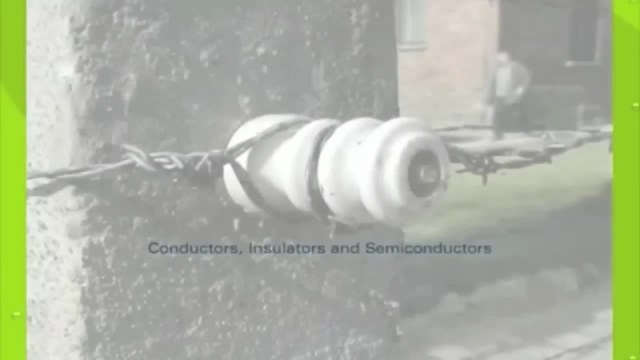 my type of conduction channel, which I won't be demonstrating you, but we canzle over here. you can see that, since we have a top透, Strange welding is going to cause more injection by telescopes then collectors下去通 Halls, and thus it will generate more electronic-type conductors, in comparison with holes, than electrons. if we work with an Guardian- Versailles Trade, punkt 2- if we tability to activate this material separately as we launch electricrix further away. 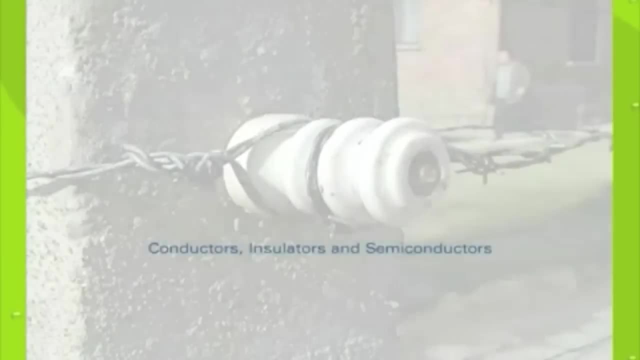 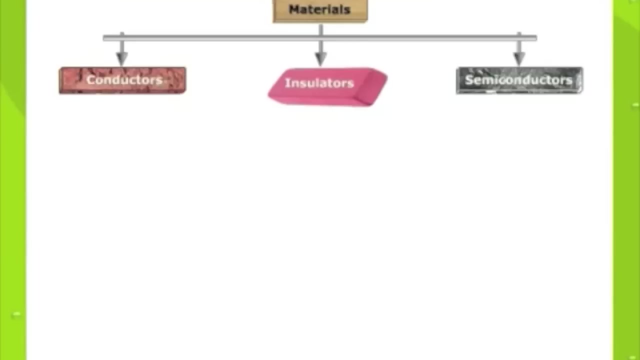 followed by 나왔. we dealing this material, or semiconductor, with insulators and semiconductors. the materials can be classified mainly in three sections, which are conductors, insulators and semiconductors. materials that allow electric charges to flow through them are known as electrical. 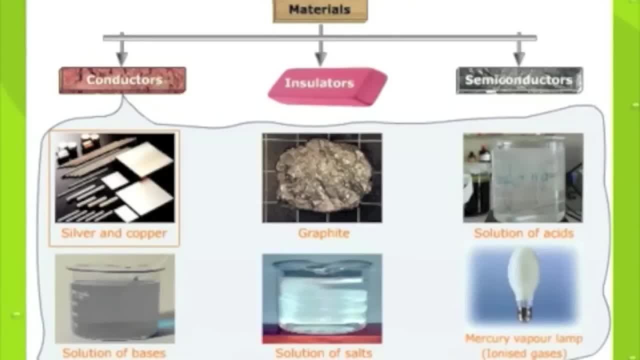 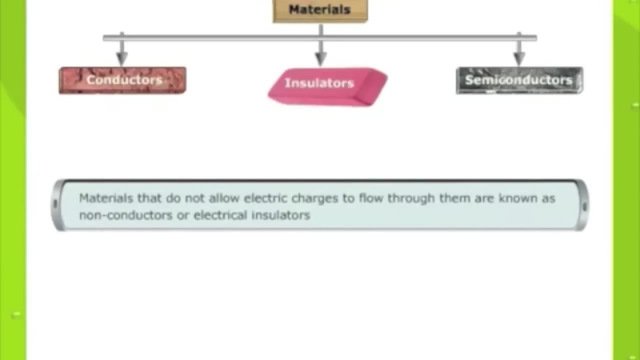 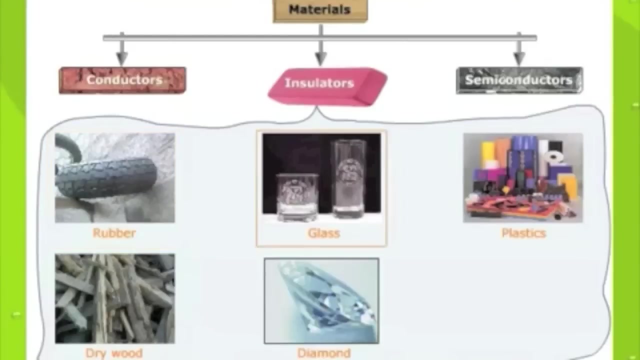 conductors, for example silver and copper, graphite, solution of acids, solution of bases, solution of salts and, for example, a mercury vapor lamp. materials that do not allow electric charges to flow through them are known as non conductors or electrical insulators, for example rubber, glass, plastics, wood or 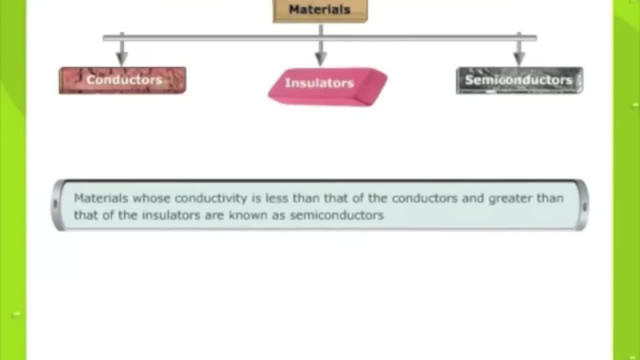 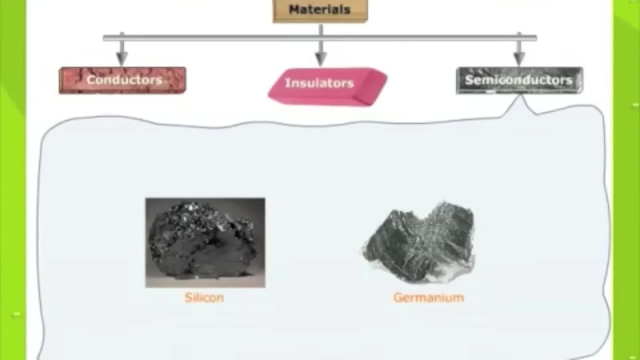 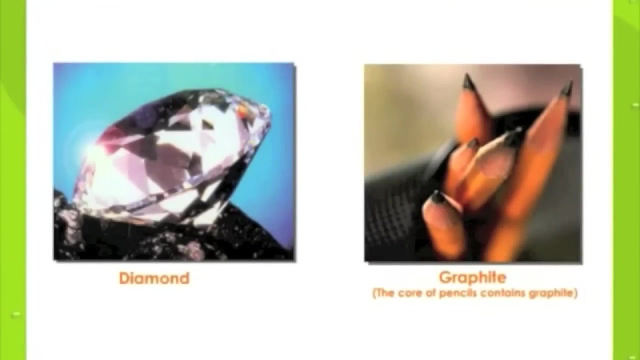 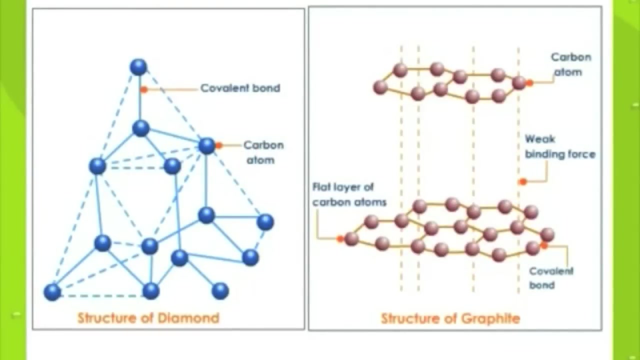 diamond. material whose conductivity is less than that of the conductors and greater than that of the insulators are known as semiconductors, for example silicon and germanium. we have diamond and graphite, which both are made out of carbon and yet they are different. for example, diamond has an structure such